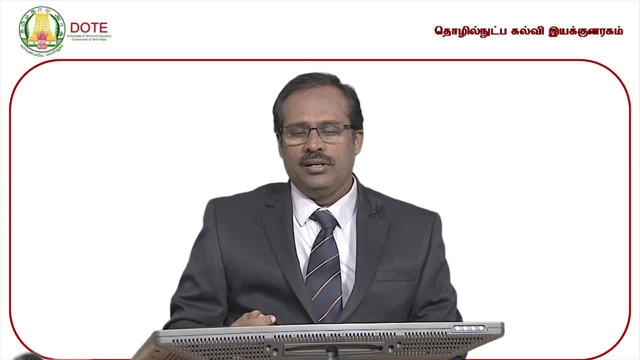 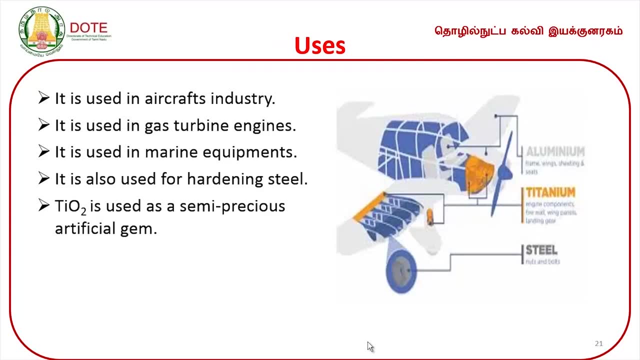 point. Then if we look at the conductivity, it is a very good conductor of heat and as well as electricity. The next one where we are using the titanium metal. The main area used by titanium is what Aircraft industry. So in this diagram, if we see that one – the yellow part will are used Every. 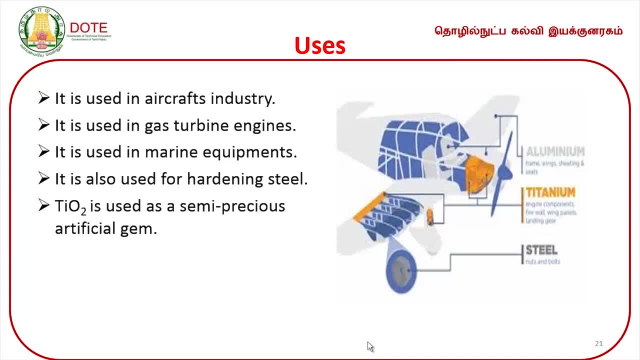 oil element is here Also. it is used in the gas turbine engines And further the special ships what they do In this case, marine equipment. We are using one of the metals made of titanium, It onw, used for hardening the scene. Titanium dioxide is also used as. 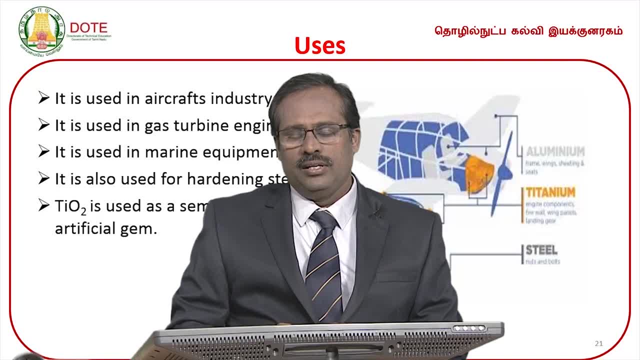 a semi-precious artificial gem – the gem we get the title in in our mythology as masters. So we have beenalt. agora In our mythology we do not have gem stone, But here we have gem state material which is used to solidify steel. This is인 shrewd stone, So we need glowing steel, which is imaged out as making 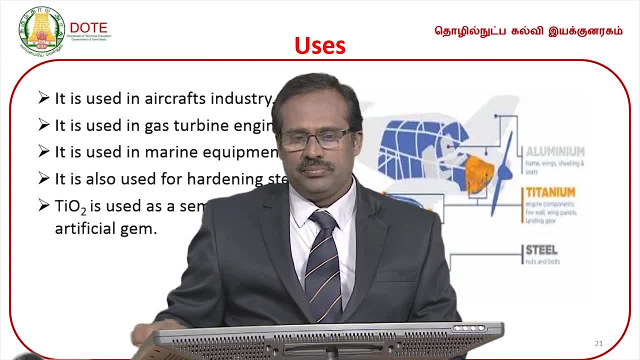 dioxide is also what one of the artificial gem of a main on the cubic zirconia, the titanium dioxide. la one of the artificial gem ma use pan ranga the navarathana karakal, la path it ping. navarathana karakal, illa me naturally karakal. artificial aum patina titanium dioxide. 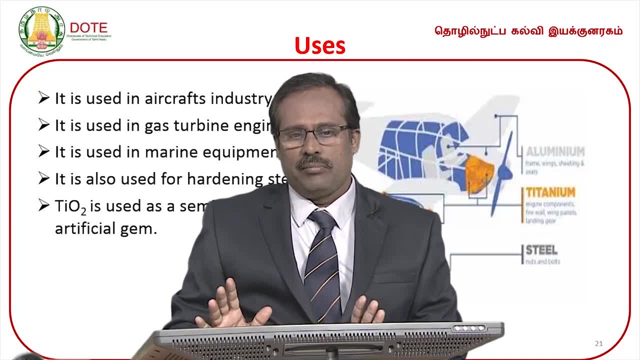 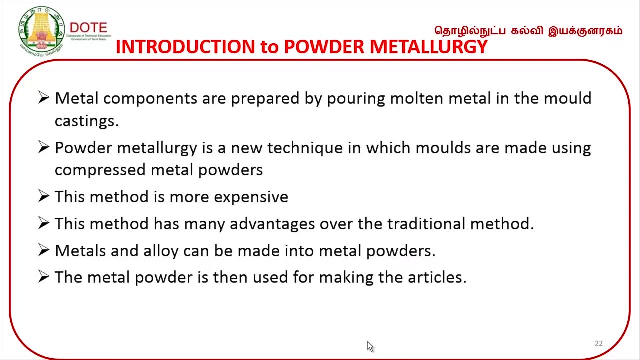 it looks like a diamond, ma, but it is not a original diamond, it is a artificial one. mainly, what edu kaha mair pan ranga na the cost wise, what very cheap that metal, that material is a very cheap one. these are some of the uses of titanium. next, next lesson, metallurgy powder. 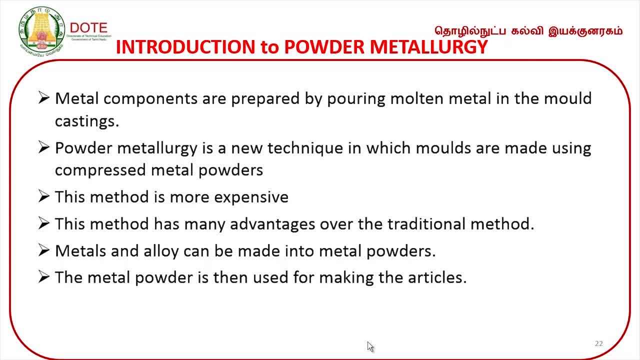 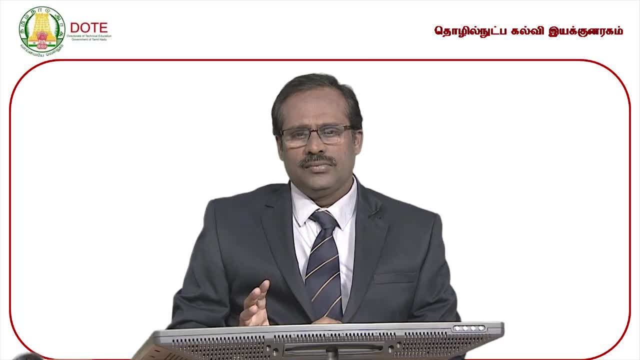 metallurgy in continuation. third unit. that lesson is a powder metallurgy normally. the powder metallurgy. tamil sunam na tool, uloho vial. the metal solid formula, thool formula, kundor for better finishing, illa me power nala idhar kundha. normally metal components. 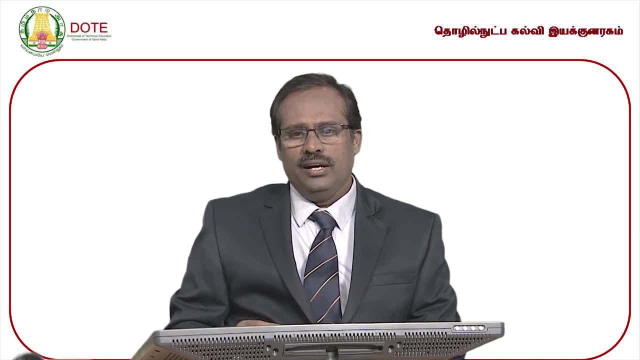 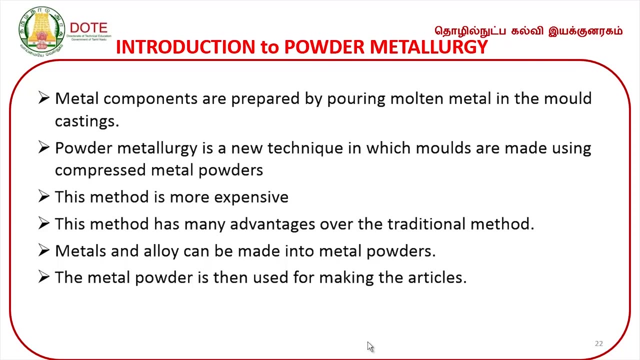 are prepared by pouring the mold and metal in the mold castings. nama ur metal a nalla urikki kaachi ur semi solid formula. oothana tham molding castings. illa la we can get a very good shapes appara powder metallurgy is a new technique in which molds are made using a compressed metal powders. 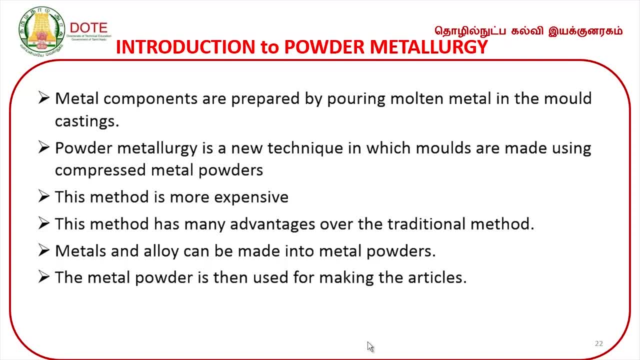 appa in the powder metallurgy. ingrati kittathri nama olden days. illa ena pannipam casting molding illa sullit pangin athala la. sometimes air holes may be what formed air bubbles in the mind illa form a chances are there. but nowadays powder metallurgy is a new technique. 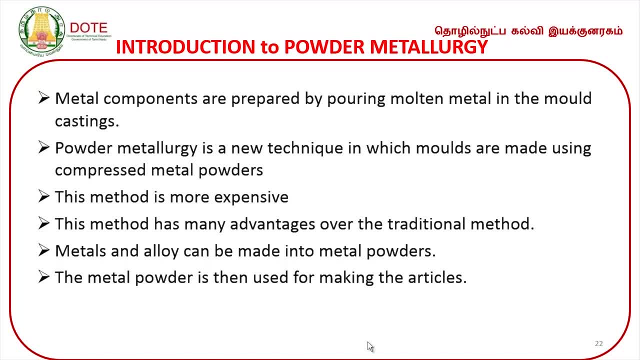 in a punta metal, odda powder, a compressed manner, la panni, we are getting a fine finishing as well as fine outlook of the things. this method is a somewhat more expensive than the olden days methods and this method has a many advantages over the traditional methods. enna. 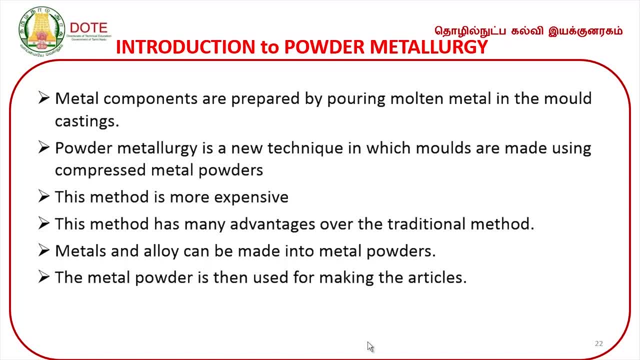 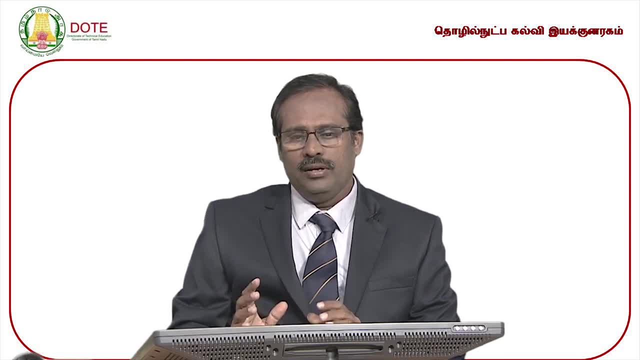 maurayana advantages. paathamna, the metals can and alloys can be made into metal powders. atha uloho mattum illa ma uloho kalaveyum nama. metal powder formula: pannumna. finishing everything will be a beautiful. the metal powder is then used for making the articles. 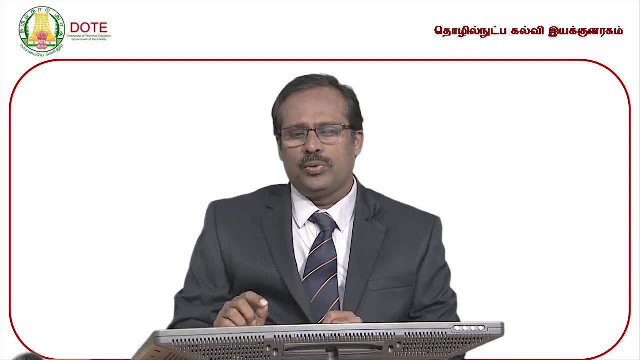 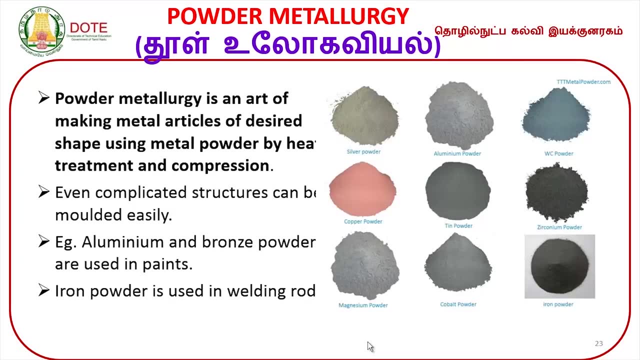 also. whatever the articles, so andamare articles, ekala, nanda, technology, use pannumna, we are getting a very, a good finishing as well as shining one maule, the powder metallurgy in a enna. what is mean by powder metallurgy? a tool, uloho veyal sorumli ya, it is an art of. 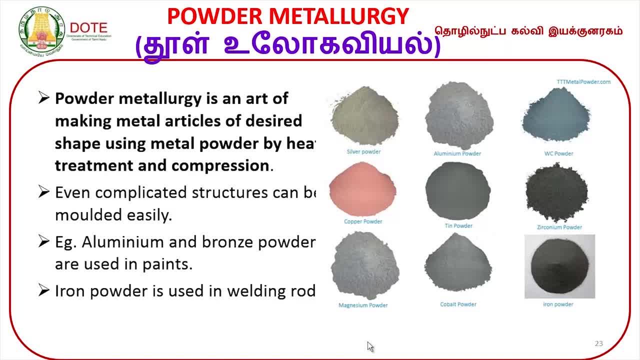 making a metal articles of desired shape- nama ke teveyana. shape maire enna. article vanaan pannikila- by using the metal powder. the metal powder is then used for making the articles also, whatever the articles. so andama maire articles, ekala nanda technology use pannumna. 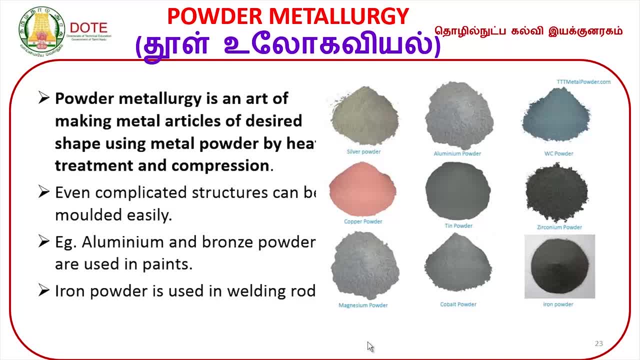 by using the metal powder, by heat treatment and compression. enna pannuram. heat treatment: nalla veppamana ithallyo compressed stage ithally, we are getting a very beautiful articles, a varudhu appa the powder. metallurgy is an art of making a metal articles of desired. 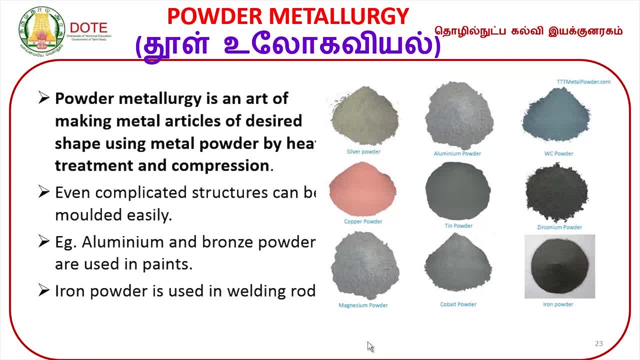 shape using the metal powder by heat treatment and compression. ithally paathamna ithally sila. complicated structures can also be molded very easily. sila edangal allana ithally kustumana atkmaar inatkmaam syilu kaana gune indana nel paratthaka ready buyer zwei up paratha darampe urte pomise. multi metal ka otra uitarane netamana. we can get a a beautiful shape. and then aluminium bronze powder are using hunting sells. iron powder is using welding rods, the tool annex- publically- how are you scene? I love governing arts place pond, wilmington, tryuldade. the 40 photographs atlo. 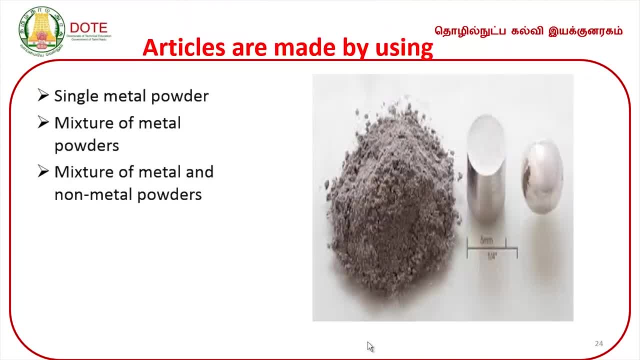 You can see that one diagram. Then articles are made by using a single metal powder. What is that? Some articles can be made with a single metal powder, or you can mix two or three metal powders and make a mixture of metal powders. 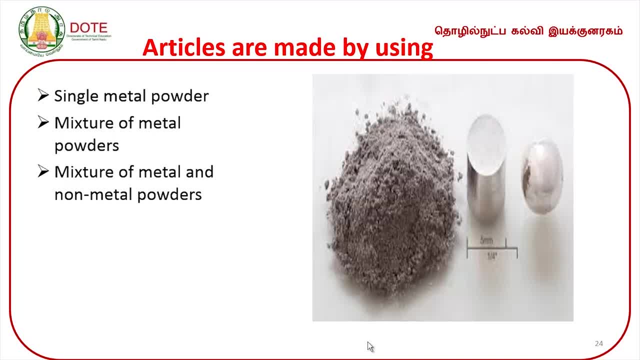 Some articles can be made with tungsten and titanium powders. Why? Because you know that the world is a mixture of two or more metals. When you mix these two or three metals, the properties of the powders are slightly modified. So if you make it in the form of powder, it is a very good one. 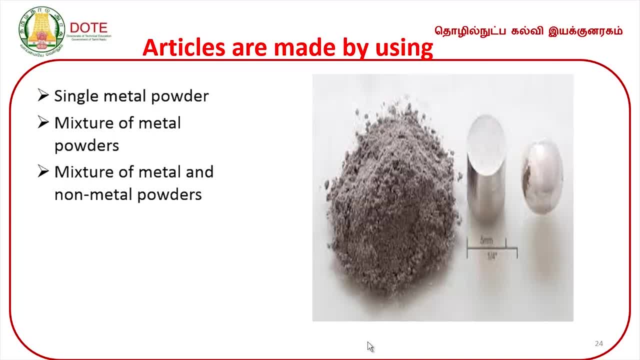 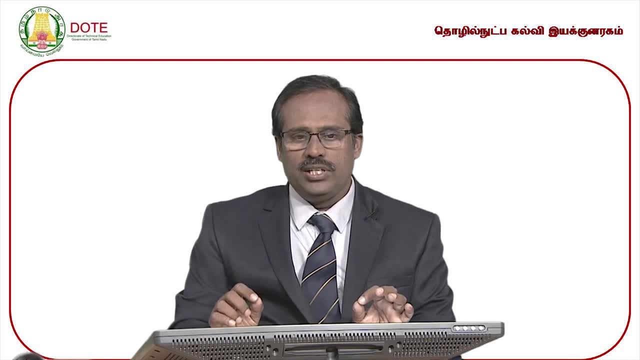 Better finishing as well as better properties may be there. A mixture of metal and non-metal powders is also possible. All the three categories. One is only one single metal powder. You can make articles like that. Second is a mixture of two or more metals. 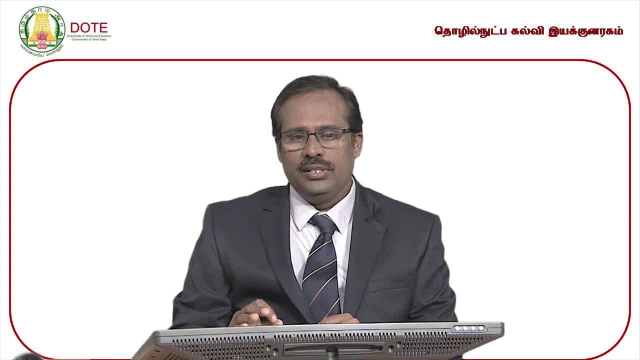 That is a mixture of metal powders. Third is a mixture of metal and non-metal powders also can be done. So if we make everything in the form of powder, Main finishing, as well as what A beautiful as well as the complicated structures can be easily made. 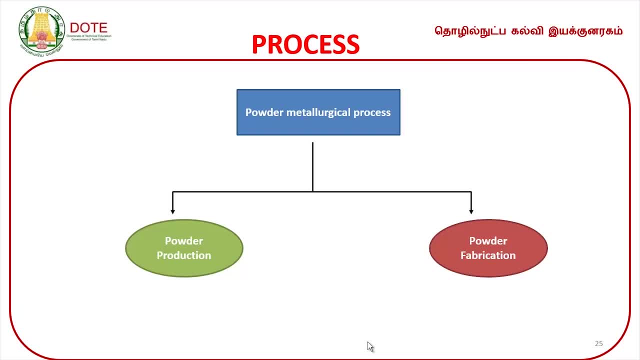 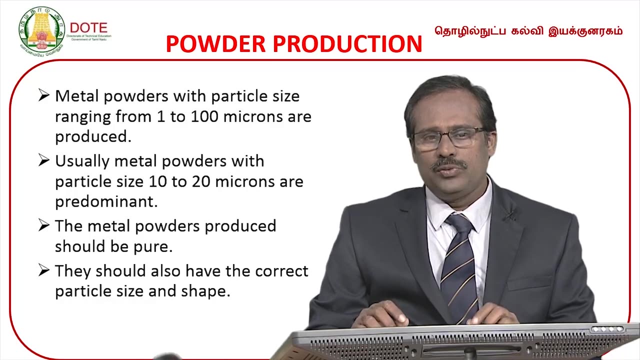 Next process of powder metallurgy, The powder metallurgical process. there are two different methods are there. One is a powder production and one is a powder fabrication. The powder fabrication we will discuss one by one. Powder production means what Metal powders with particle size ranging from 1 to 100 microns are produced upon the metal. 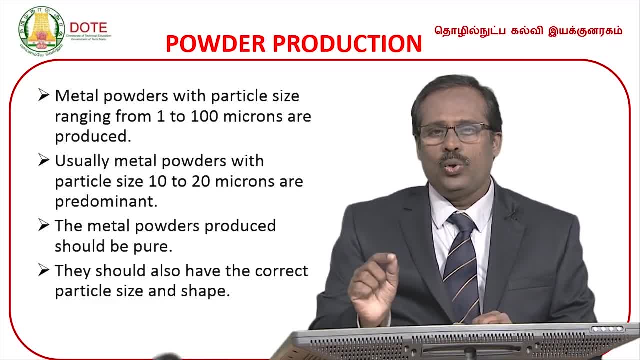 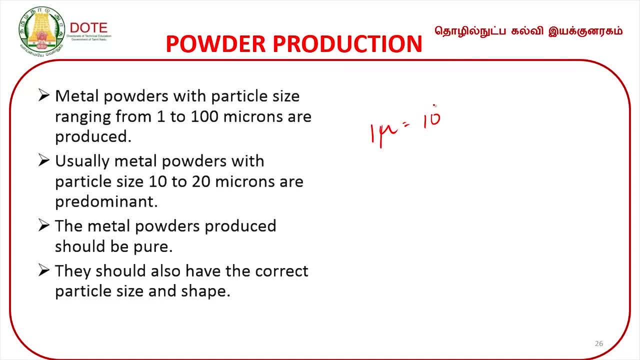 powder form, If it is a 1 to 100 microns. 1 micron is equal to 10 to the power of minus 6.. One micron is equal to 10 to the power of minus 6.. So this way, 1 to 100 microns, we can produce. 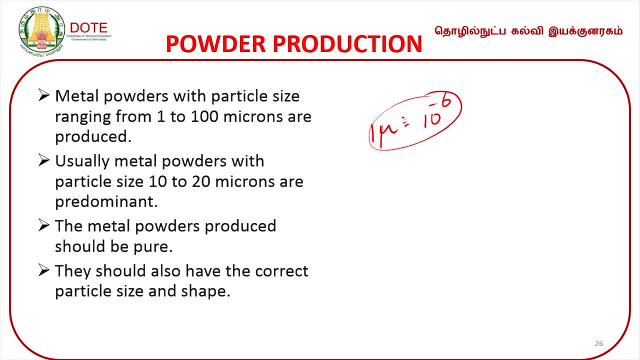 Usually metal powders with particle size 10 to 20 microns are predominant. So in the powder production the main thing is 10 to 20 microns. is what Predominant, It will be good. So the powder produced should be pure. 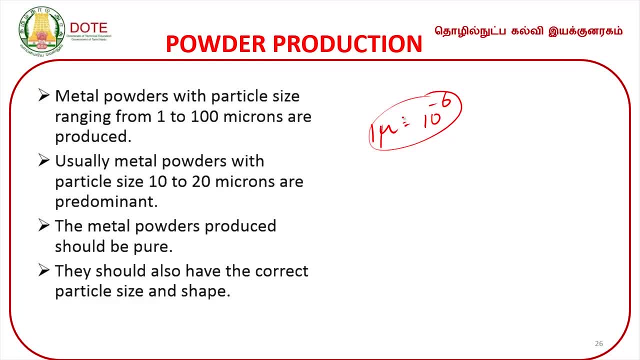 They should also have the correct particle size and shape. So for the powder production method we are getting that what The metal powders should be in a pure form as well, as the particle size and shape will be correct Then preparation of metal powder. 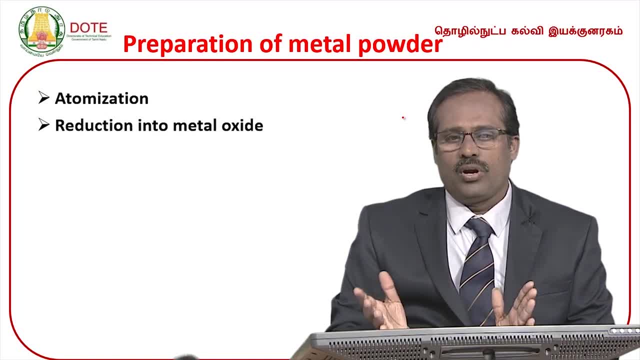 How can we make it in a solid form? It can be iron or it can be a rod or any other form, So how we can convert into metal powder form. There are two methods for that. One is the atomization method, Another is a reduction into metal. 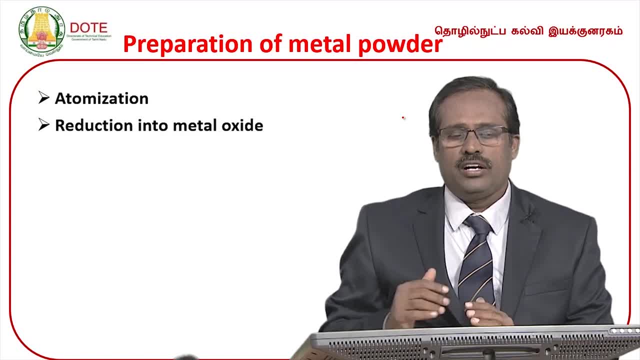 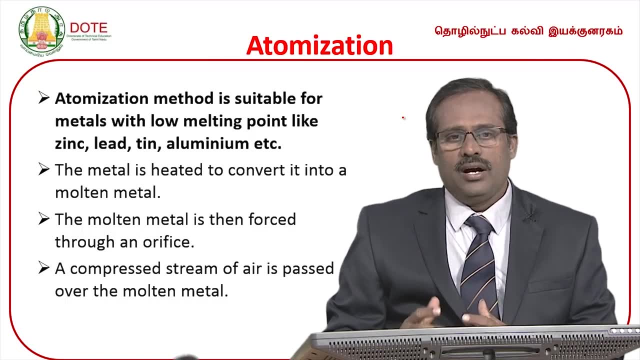 Okay, In the two methods we will discuss one by one Atomization. In Tamil it is anuakkal murai. Atomization method is suitable for metals with low melting points. So in metals we are having a lot of metals. 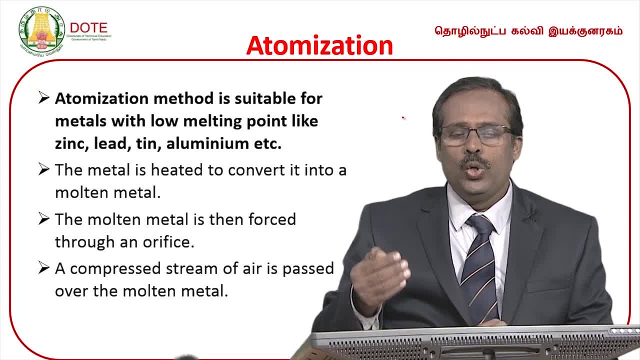 Like zinc, copper. Even if there are lot of metals, which metal is in low melting point? we can choose the atomization method. So you saw what metal it is. The metals in low melting point- zinc, lead, tin, aluminium. zinc, lead, tin and aluminium in the metals are suitable for. 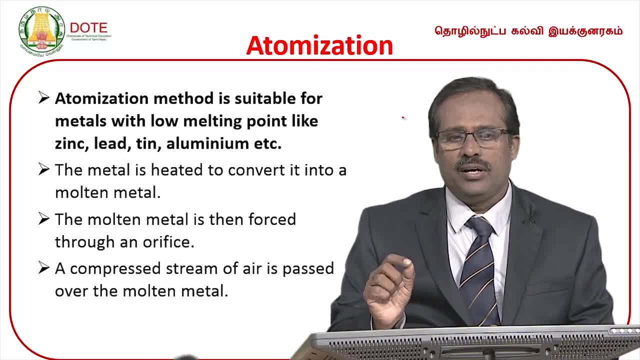 atomization method. Because of the property called low melting point in the metals- very, very low melting point- we are choosing for atomization methods. Second one: that metal is heated to convert it into a molten metal. The metal will be converted in the form of what Semi-solid? 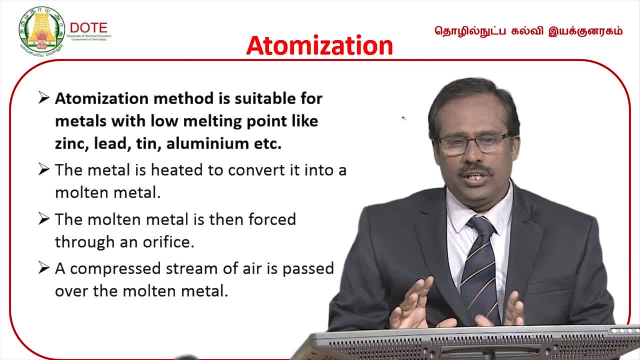 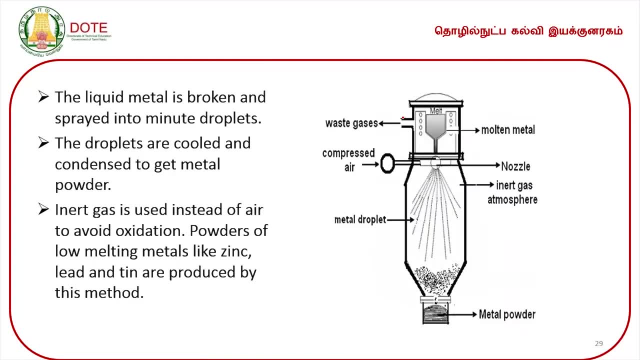 formula that is called molten metal. The molten metal is then forced through an orifice In this diagram. in this area only we are having that molten metal that is, at a particular temperature. The molten metal becomes what Converted in the form of semi-solid form. That is what 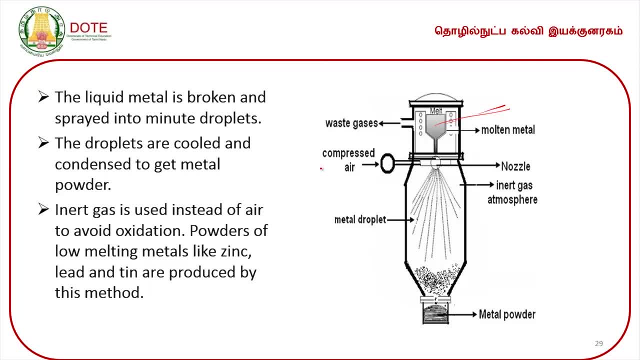 we call molten metal, And the molten metal is there. Through this we are passing the compressed air and the nozzle. Then inside the furnace we are having a inert gas atmosphere. Why we are choosing inert gas atmosphere? If it is the air passed, what will happen? 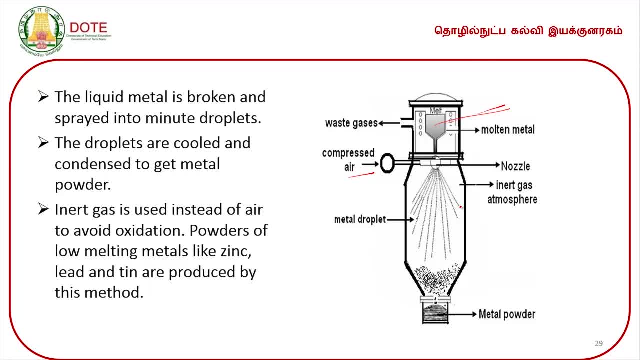 That air containing some oxidizable substances Oxidation have a chances of oxidation. Oxidation field has chances are there. That is why what we are doing is using a inert gas atmosphere. We are using an inert gas atmosphere. Irinet gas is an interactive 47 channel system. 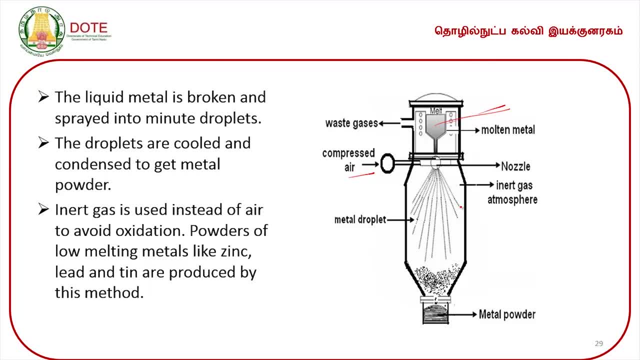 Now here you can see the ír witnessed here- WhenMoulònPowderWautemold small, small droplets are converted. droplets are converted, that will be follows a pieces: small, small particle size. that is, a metal powder for metal. metal powder for metal. 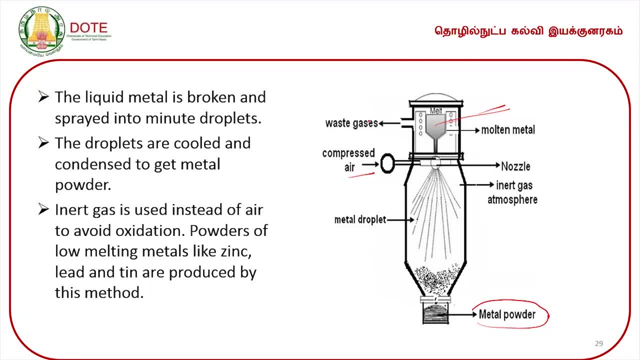 If any gases- unwanted gases or waste gases that will be exit in this way. So by the liquid metal is broken into minute droplets. the droplets are cooled and condensed to get a metal powder, inert gas. we are. we are using for what? to avoid the oxidation purpose. So 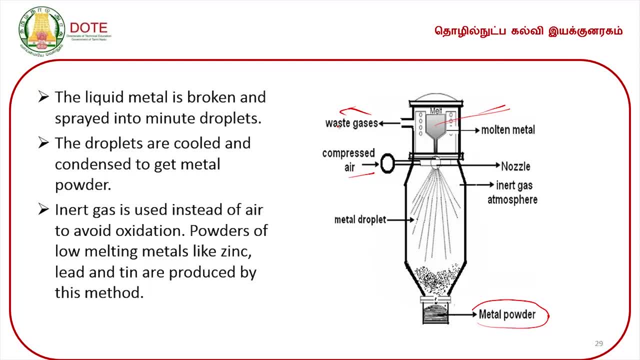 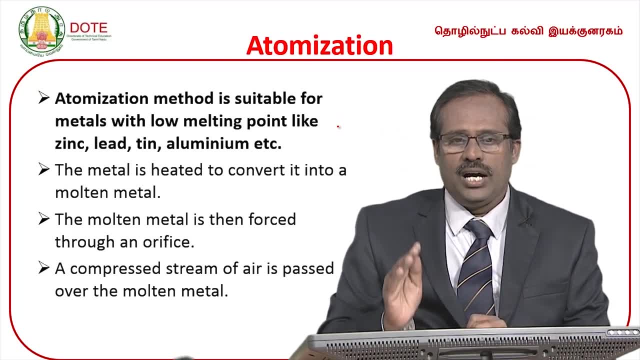 oxidation powders of low melting metals like zinc, lead, tin are produced by this method. So the atomization method? what is the atomization? atomization method is used? suitable for what? metals which are having low melting points, like zinc, lead tin, aluminum, etcetera. So 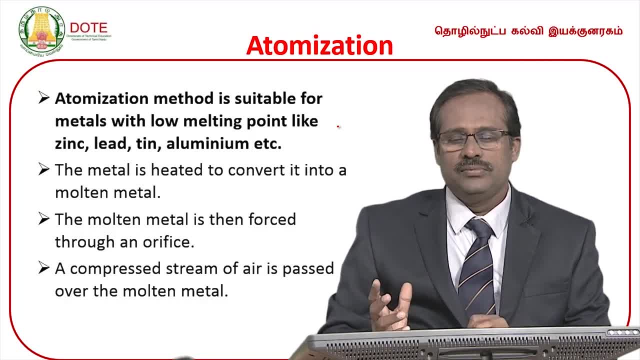 the metal is heated to convert it to a, to get a molten metal. So this is the second stage, a semi solid formula: convert the first step. Second step: the molten metal is what then forced through an orifice. orifice is a small pin drop size. 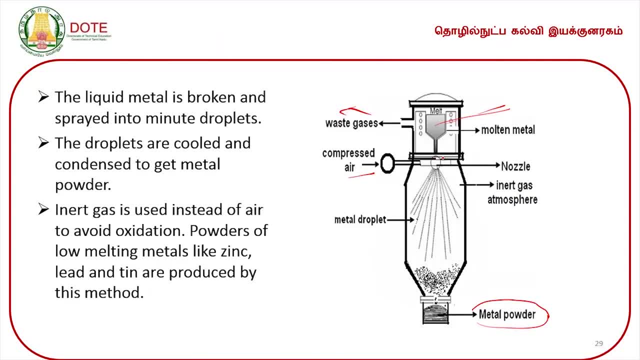 you have to think about the small nozzle size, small pin hole size through that we are passing the molten liquid When you pass the compressed air, and then what will happen? the molten liquid level, or droplets, are converted. it will be what come down as a powder form. Then 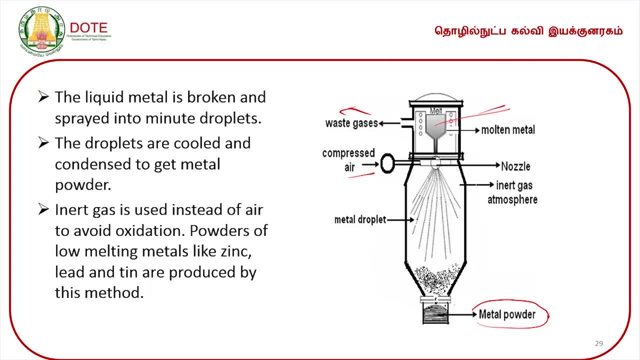 the droplets are cooled and condensed to get a metal powder. So in this purpose or in this method, we are using a inert gas to avoid the oxidation. So the atomization methods we can choose, the metals like which are having very low melting points, like zinc, tin, lead. 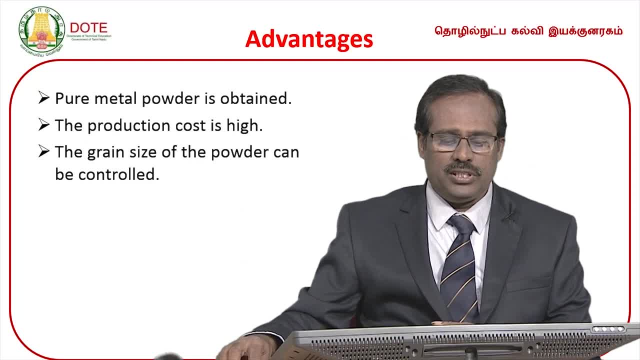 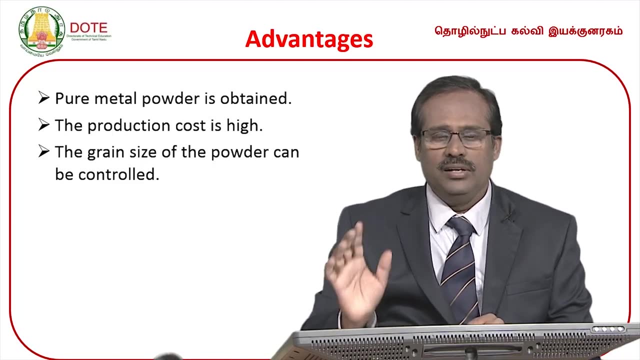 etcetera. Then what are the advantages of this atomization method? First one: pure metal powder is obtained. second one: the production cost is very high. Third one: the grain size of the powder can be controlled. that means, whatever the microns we want in the atomization method, we can do the things. 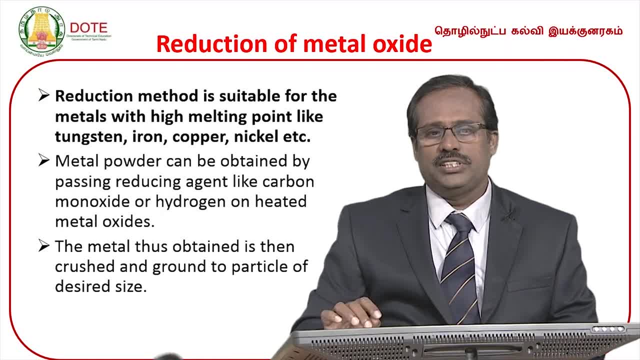 Next one, reduction of metal oxides. first one is atomization method. second one is reduction of metal oxide methods. What is the reduction method? The reduction method is suitable for the metals with the high melting point, like tungsten, iron, copper, copper, copper, copper. 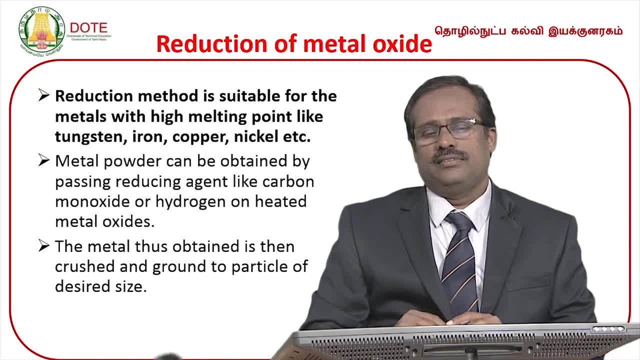 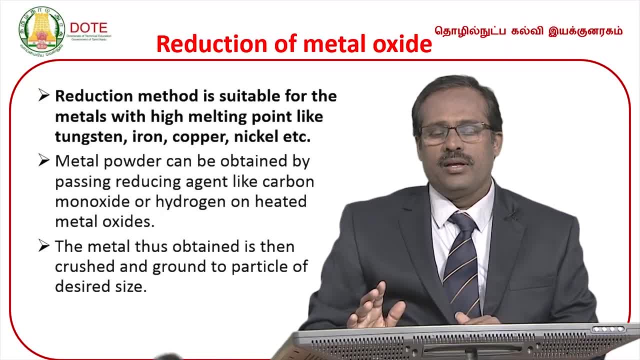 low melting point. Now in the reduction method we have to choose the metals which are having high melting point. What are the metals? tungsten, you might have already seen in the lecture, does not matter, but for tungsten there is a melting point which is 877 Kelvin, 77 degree. 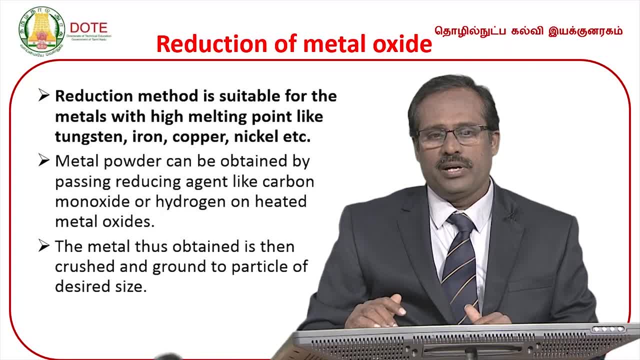 centigrade, So that is the very highest temperatures. There is definitely power dissipation in tungsten and so there is a regulation based on that amenity. So andamer metal like iron, copper, nickel is allow the reduction metal. that is a best. 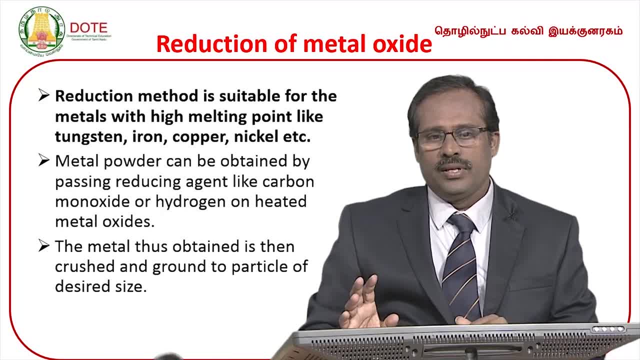 method for the convert into powder form, So we will discuss one by one. Metal powder can be obtained by passing the reducing agent like carbon monoxide or hydrogen on heated metal oxides. The metal obtained is then crushed and ground to particles of desired size. nama. 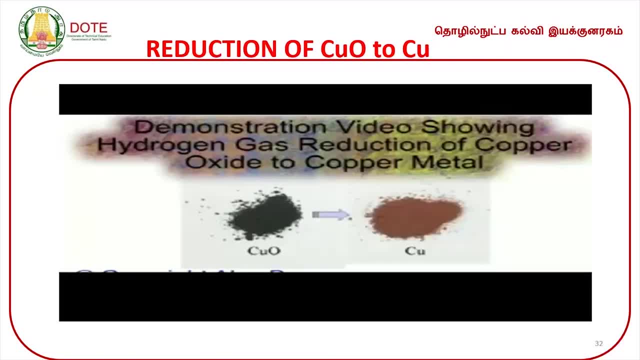 ki enna maari particle size devi aadhappadi nama eduthukula The reduction of metal oxides, say for example, copper oxide to copper. ur chinna video molemma eppudi nama metal oxide here nama taken enna eduthukula nama copper oxide, eduthukula copper 2 oxide, or you can. 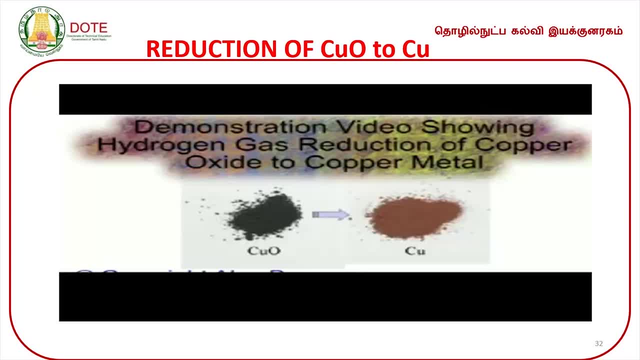 say cupric oxide, which is normally black in color. Aadhi eppudi copper a convert. aadhum pavadhu copper color. unkalu paathir pinga copper tamiram ur maari reddish brown color la rukum. 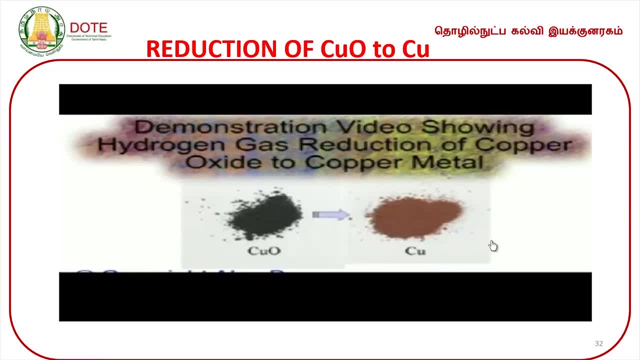 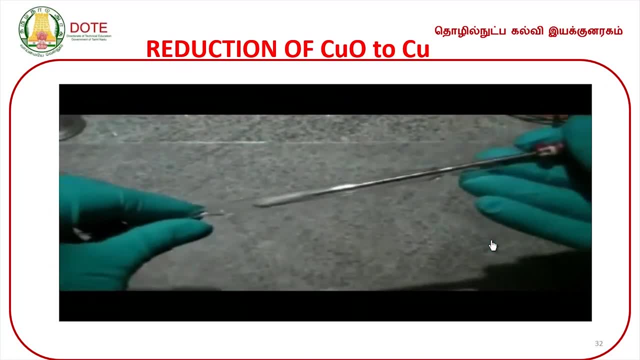 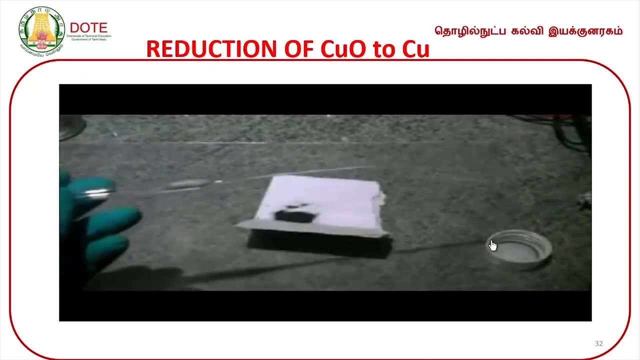 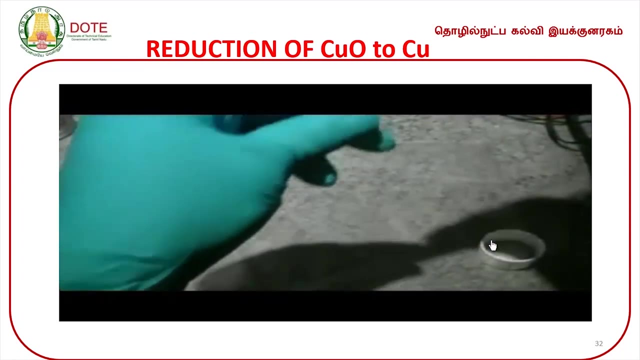 And the stage eppudi convert aadhum parung ur chinna video molemma The experiment eppudi sandaam parung ur chinna tube la we are filled with what? cupric oxide, which is a black in color, karuppu color, la rukum salt aadha cupric oxide formula. 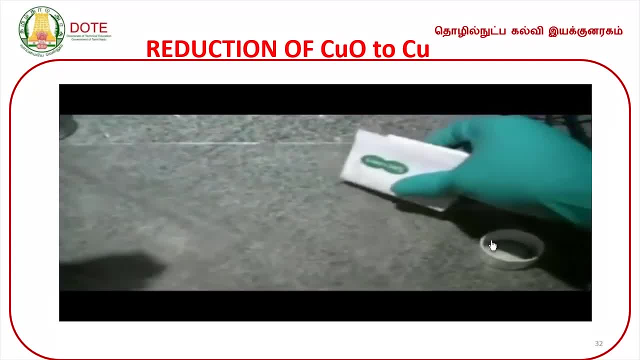 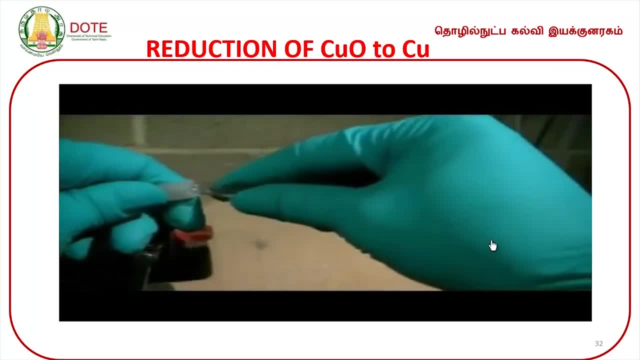 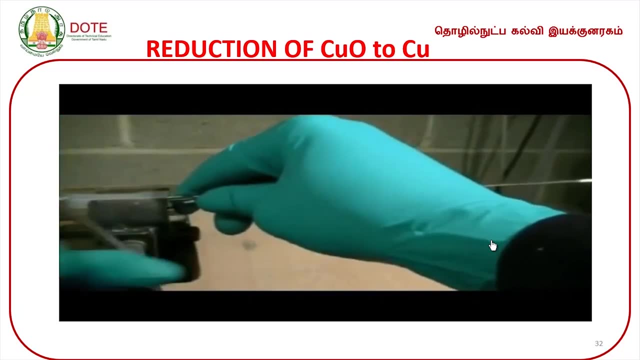 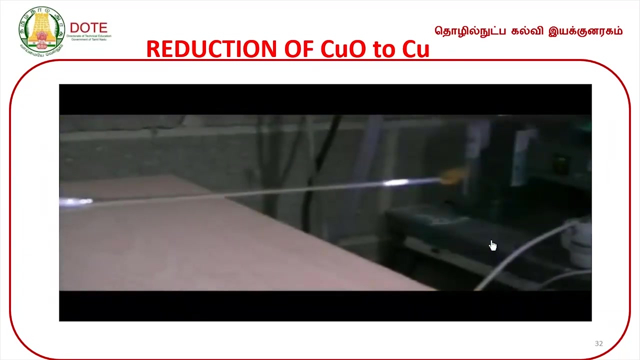 is CuO aadha, aadha la fill panittu. I will fill panittu hydrogen which reduce panuram Hydrogen gas fill pani. we are reducing the things Just on heating. that will be slowly reduce to give copper, just on heating. So 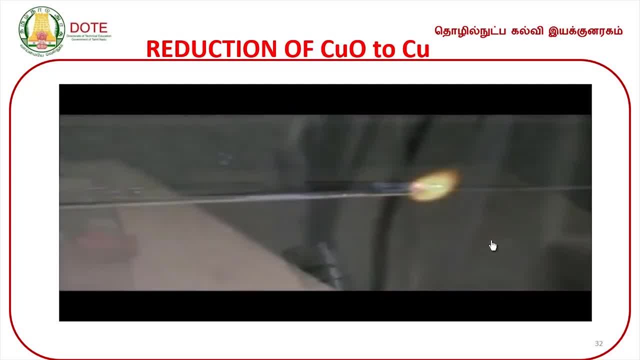 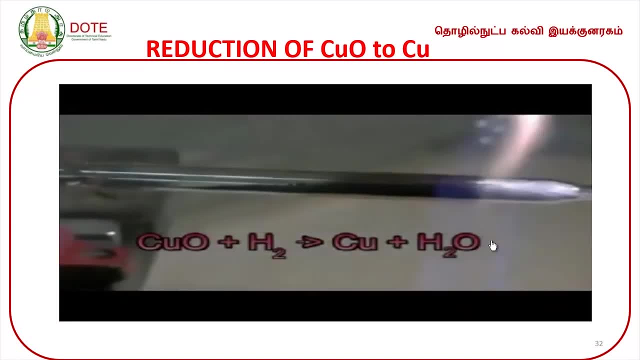 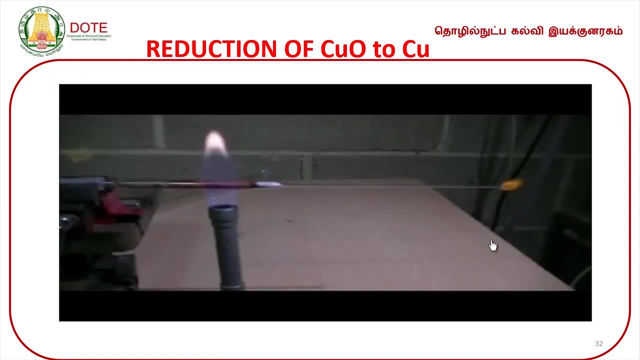 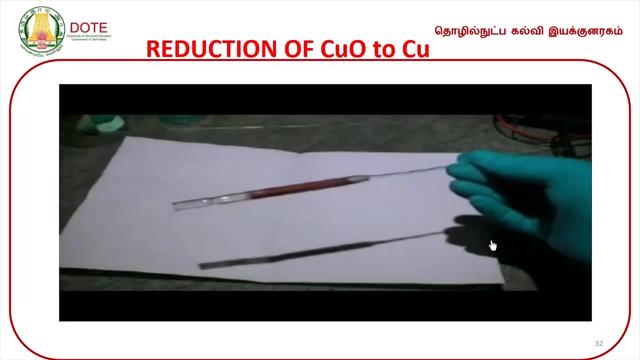 Finally, when we take it out, look at its colour. what we have added is a solid in black colour that is a cupric oxide. hydrogen is passed. it gives a copper metal and water. When it is heated well, it is fully converted to copper. 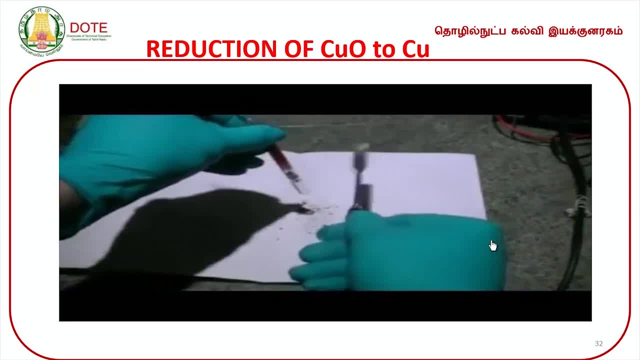 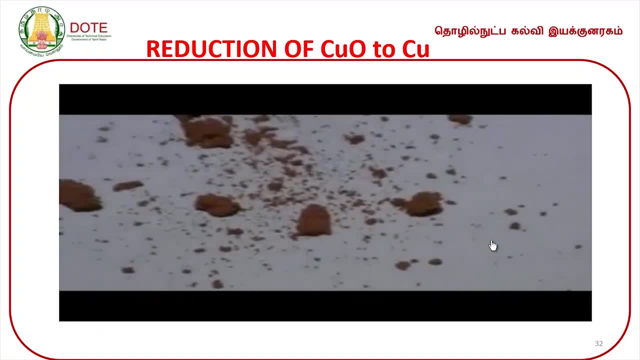 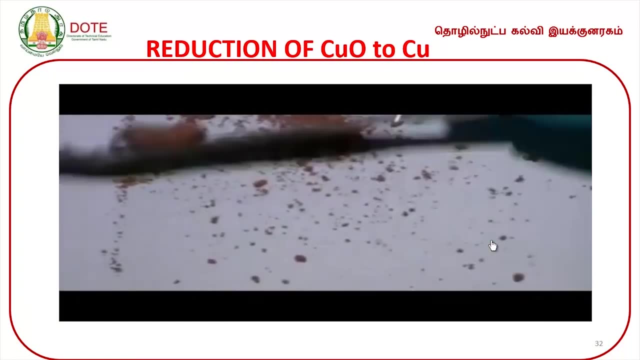 See the colour of the metal pieces. it has come in the form of powder. See the colour. it will be a reddish brown colour. that is the colour of the copper metal. We have added black colour. If we reduce the hydrogen powder, we are getting a reddish brown colour solid, which is a copper. 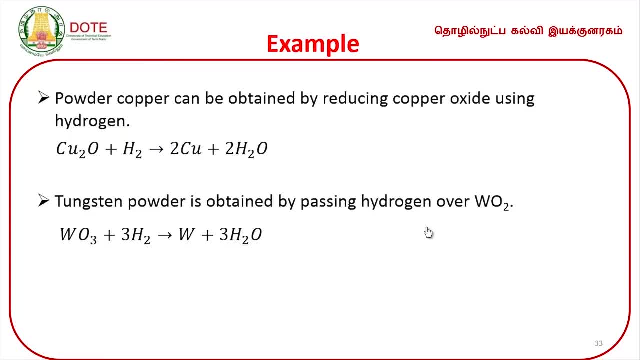 metal. Next, I will give you an example of reduction method. Cu 2 O plus H 2 gives Cu plus H 2 O. we have seen this. The another one is a tungsten powder is obtained by passing the hydrogen over tungsten oxide. 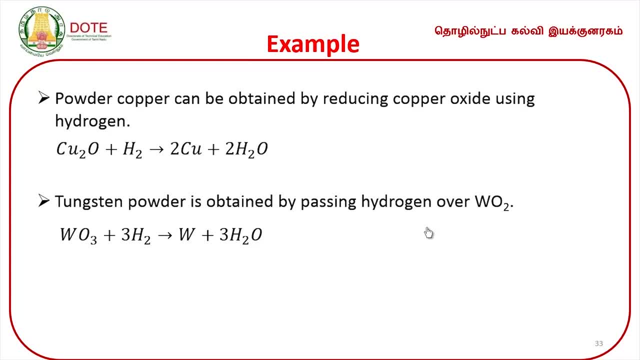 See the W O 3 plus 3 H 2 gives W plus 3 H 2 O. We are getting a tungsten powder, Tungsten powder format, So in this one it should be a tungsten oxide. These two are examples, for we are converting the powder form of metals by reduction method. 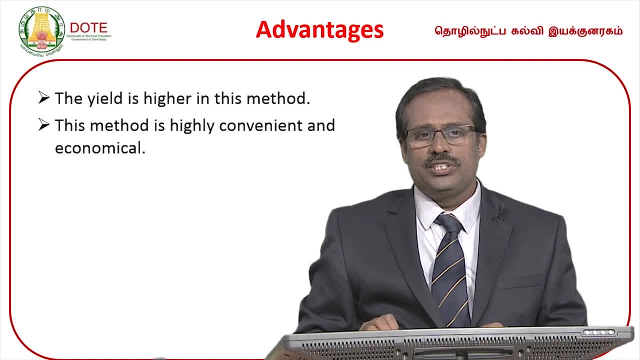 What are the advantages for this reduction method? First, one is a: the yield is higher in this method, Then it will become pulsfect. The yield is what Higher in this method, Then highly convenient and economical method. These two are the main advantages of reduction method. So one is a: nareya yield kada kithu. 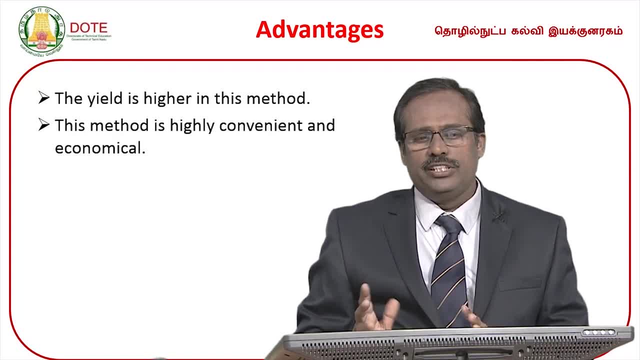 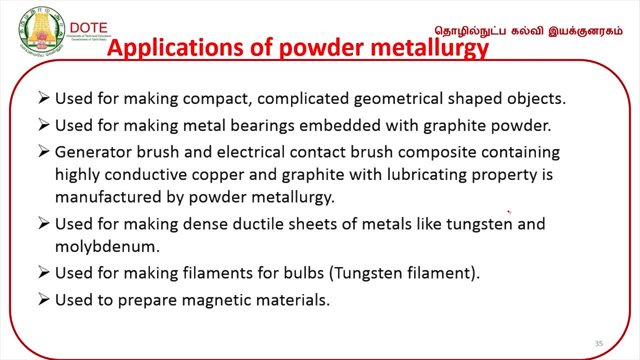 Renda aadhu economically cheap, highly convenient or easy to follow Aaduthatha. what are the applications of powder metallurgy? Ippan the tool ulohaviyaala engangal laama paayanpadathula, Engangal laama paayanpadathuna. that will be what More easier. 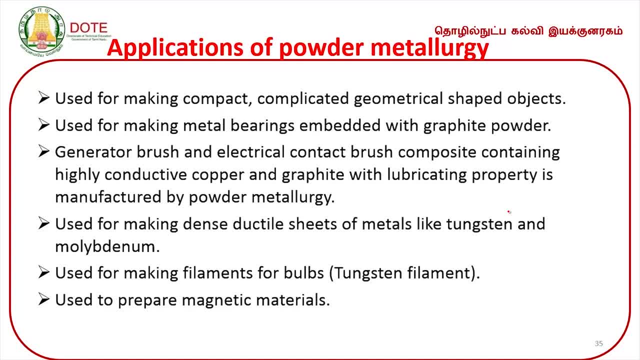 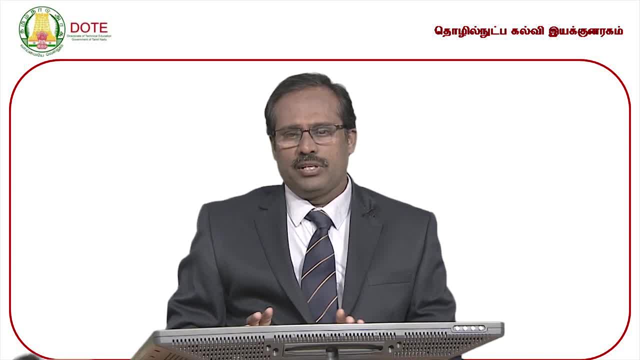 First one used for making a compact, complicated geometrical shaped objects. Uru sila amipigal geometrical shapes ilan pathingin singa vithyasam, vithyasam na amipigal laan rukum po adhula laan sadharna traditional methods, laan molding, laan pannum po. we are 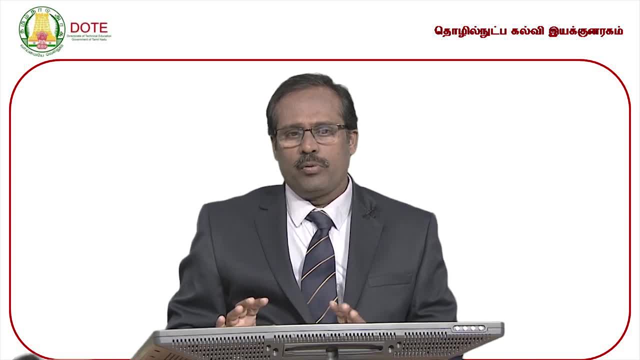 not getting a very good finishing, But in this powder metallurgy technique laan pannum naan, singa powder formula laan itithu metal itithu pannum naan- we are getting a very good structures, even the complicated structures also. 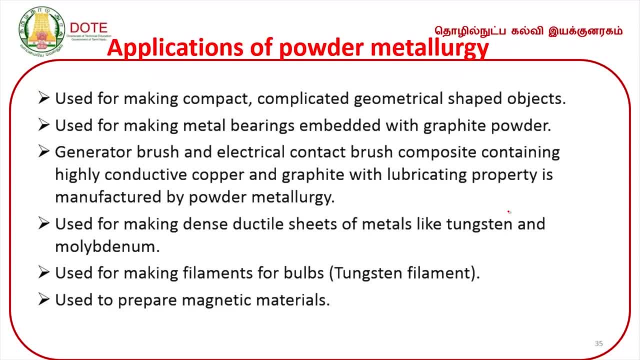 The another one is a Aadhu. Aadhu, next one, making for metal bearings embedded with a graphite powder on the metal bearings. Aadhu, next one. generator, bush, sorry, generator brush and electrical contact brush. composite containing a highly conductive copper and graphite with lubricating property is manufactured. 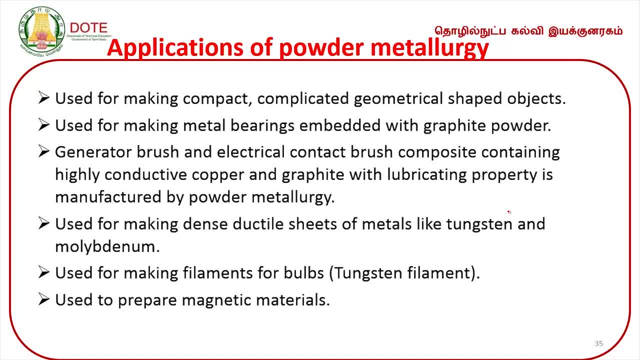 by powder metallurgy. So main lubricating property is what very important in this aspects. The next one: the powder metallurgy in all are used for making a dense ductile sheets of metals like tungsten and molybdenum. ductile means we can make into sheets. we 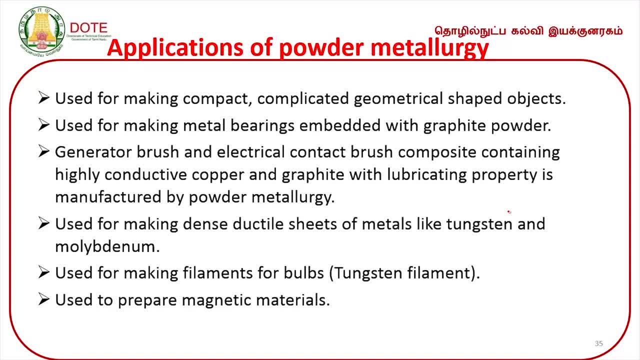 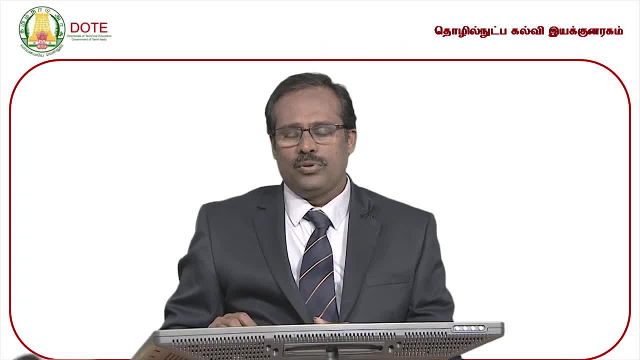 can apply this method. Another one used for making a filament for bulb means nowadays we are having a LED bulbs, but in the olden days- that is what this is, 10 or 18 years back- we are using a tungsten. 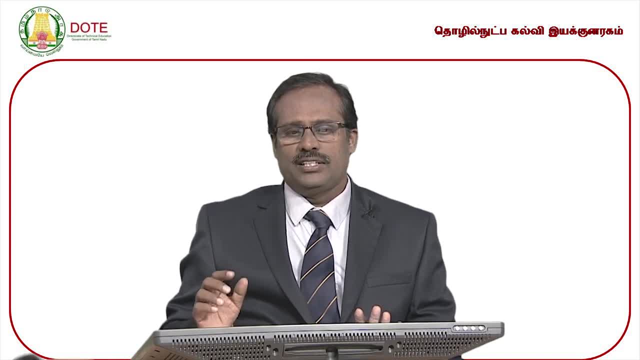 filament bulb, one ball bulb, or cool liya, actually filament on the tungsten filament. I am used to have it in myLife Now In the ghost. the main reason is what high melting point then it is also used for to prepare a magnetic 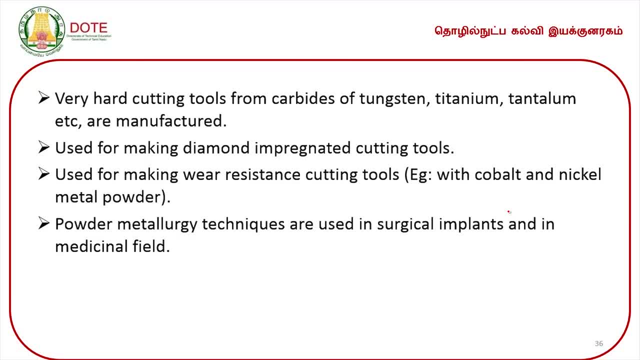 materials and also it is very hot. cutting tools from carbides or tungsten, titanium, tantalum, etcetera can also be manufactured. and also it is used for what? making a diamond impregnated, cutting tools of a marble cut up of stones. we are using that. what industrial diamond. 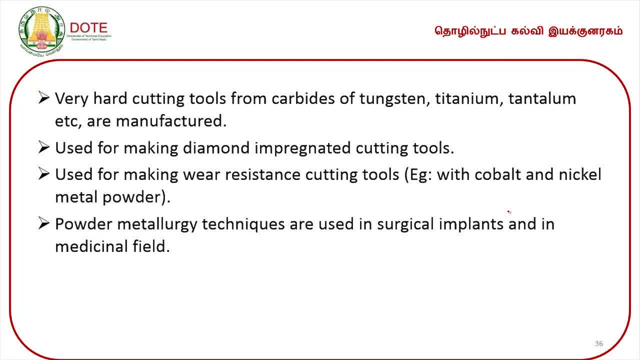 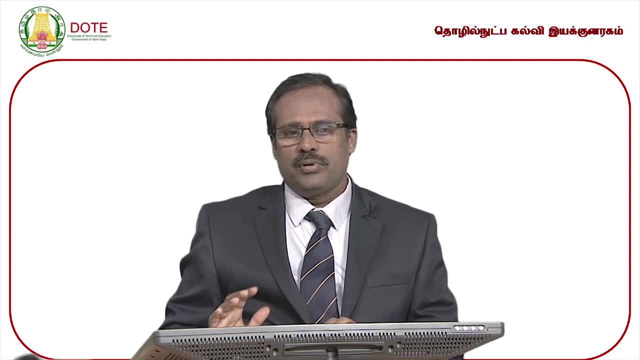 and the industrial diamond cutting tools. we are using what this type of powder, metallurgy, timbre metal and industrial diamond? ok, matala steel plate. that is what diamond impregnated tools used for cutting the cut up of stone or marbles. you are using the impregnated diamond. 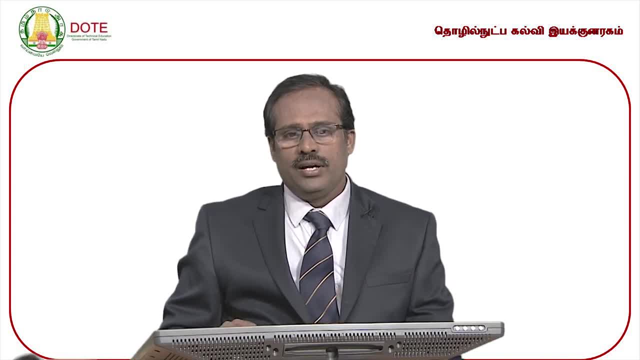 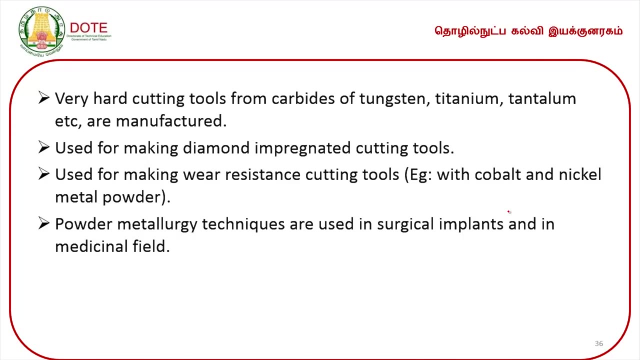 tools. next, it is also used for what? making the wear resistance cutting tools, cutting tools upon your metal mix money, copper, copper, copper, copper metal powder. we can use for wear resistant cutting tools. The powder. metallurgy techniques are also used in the surgical implants and in the medicinal. 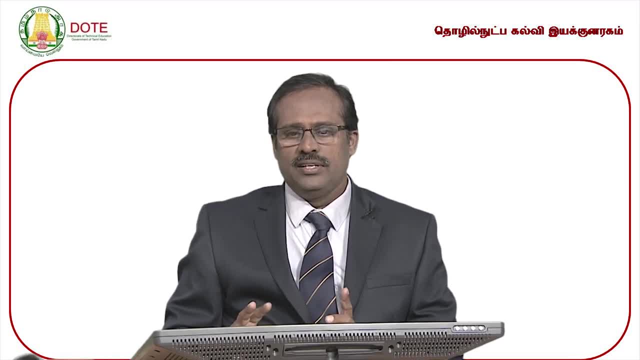 field, also So surgical. what instruments? like the first optional use material all along, they are using this type of powder metallurgy technique to get a fine finishing, as well as what with good quality. Not only that, what a surgical implants or implants, and also in the medical field, And this particular lesson length. 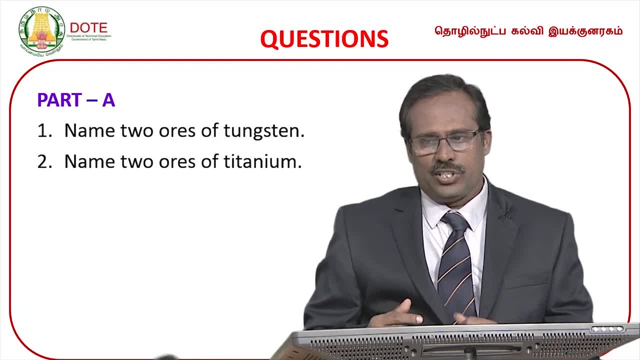 enna maari questions. kekala Porn lecture le nama: extraction of metals. paathom aadha le sella question answers. discuss panle. So ipa aadha le discuss pande. we will continue this one. In the extraction of metal le we can ask questions like what? two more questions? 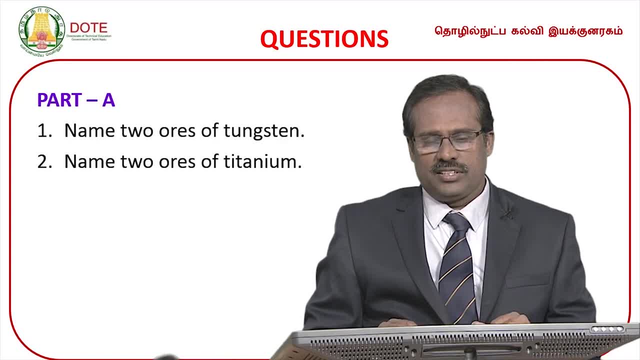 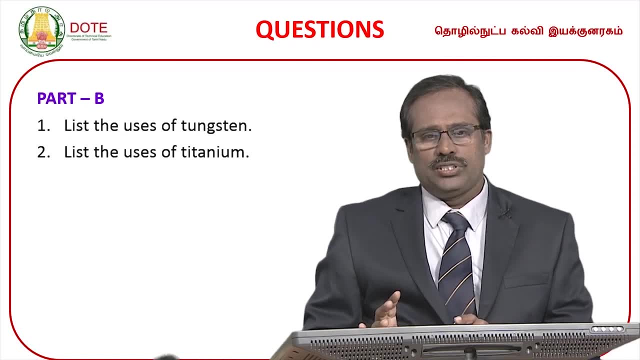 le. what are the ores of tungsten? what are the ores of titanium? Ok, The part b, that is a, three more questions. list the uses of tungsten, list the use of titanium, or what are the ores of titanium. also, they will ask In part c, five more questions. 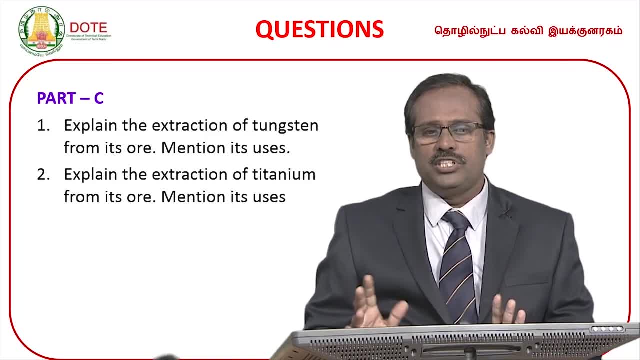 explain the extraction of tungsten from its ore, mention its uses. explain the extraction of titanium from its ore, mention its uses. So in the lesson le extraction of metal, le irukkura, there entire two questions sa, one extraction of tungsten, one extraction of titanium. So any one may be ask in the 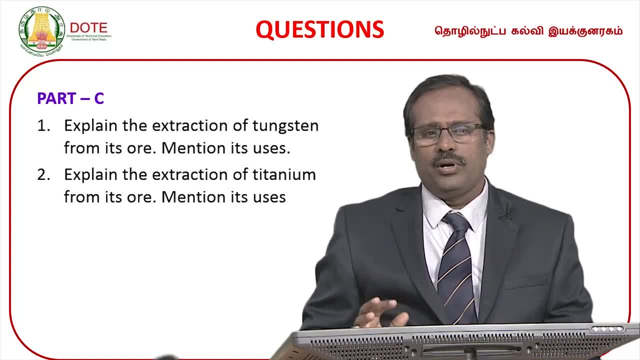 five more questions. So in the part c le. that is very important. So nama erkha ne soli rukkuma. So if it is a on the five stages, in cover pane you have to write the answers. If you are writing only the equations, they will give only a part mark, only two marks. 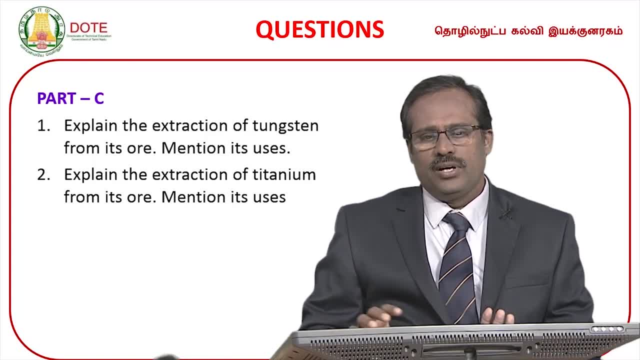 diagram, one mark in the manner they will give the how to what evaluation schemes also there. Apri five marks. you anana all the five stages with the correct equations you want, right for extraction of tungsten and the extraction of titanium, and they uses one or two uses. 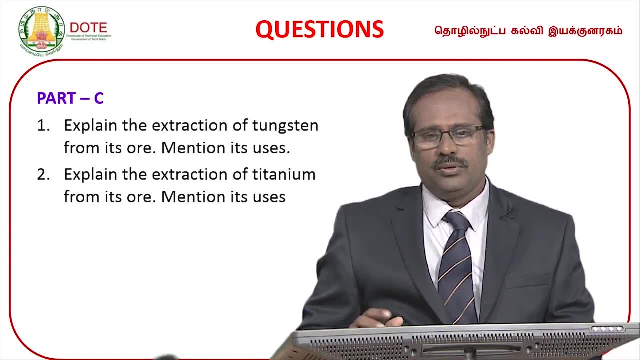 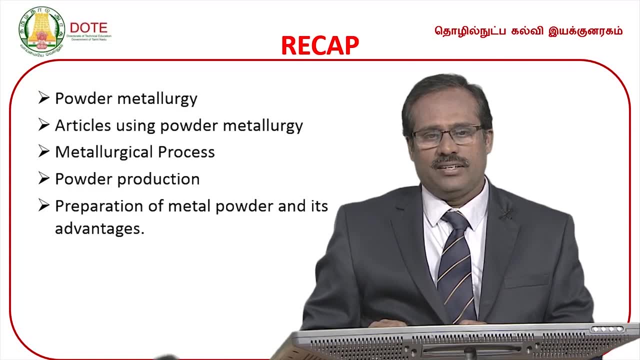 the key: le kudukkuma na mark karanya 2 uses any two mark so you can write very easily this: questions In the powder metallurgy we are. would do the recap or summarize the lesson whether metallurgy in what is mean by powder metallurgy what? 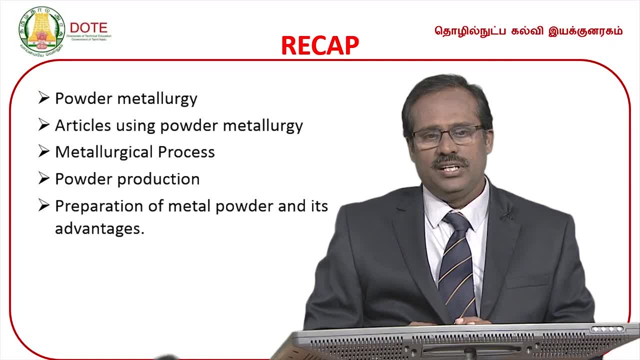 are the articles 有 energy, then the metallurgical process. The metallurgical process: we have seen two methods. One is metal production and metal fabrication. Among the two processes, we are having powder production methods and another one is powder fabrication methods. After that, we are having 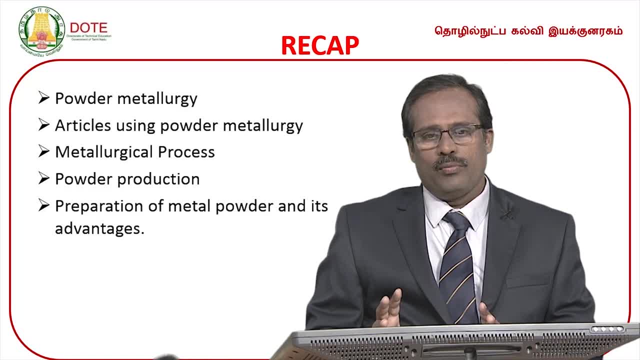 two methods of producing the powder form of metal. One is the atomization method and another one is a reduction method. In the atomization method, can you remember that one? So the atomization method, if you pass through a pinhole size, that is a orifice, small orifice. 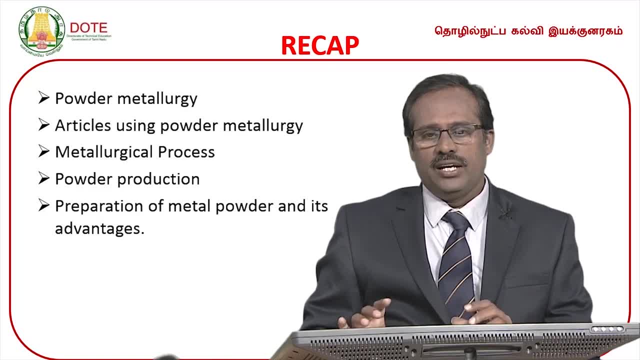 if you pass that one and compressed air is passed in an inert gas atmosphere, that will become a tiny droplets form and on condensation it will be what? Powder form. That is the atomization method, The reduction methods. You take some metal oxides by using some reducing agents or you can what? By either use a hydrogen. 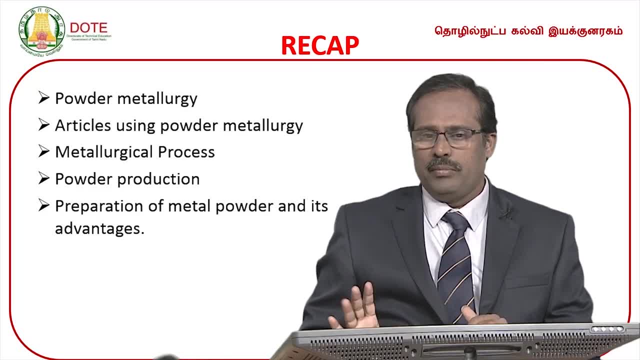 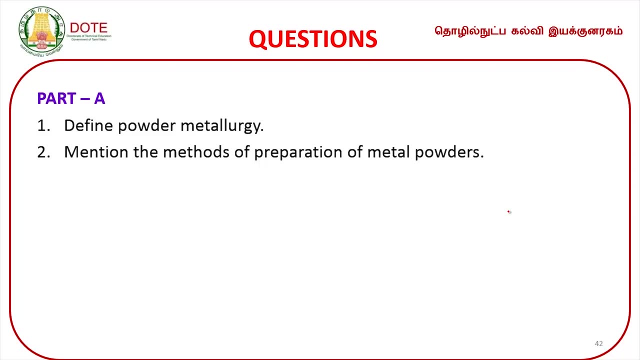 or carbon, whatever things. it will be converted to use a corresponding metal. That is a reduction process. Finally, the preparation of metal powder and its lot of advantages. There are various advantages are there In this powder metallurgy. what type of questions may be asked In the part? 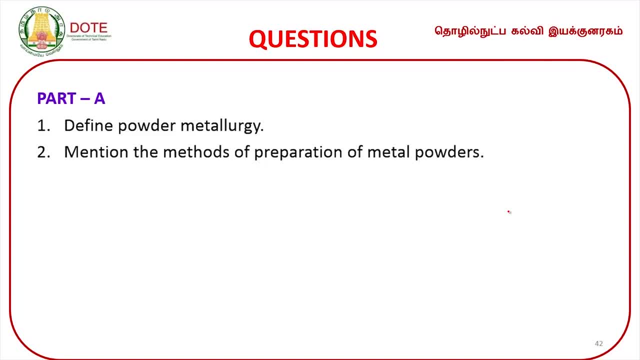 A, a defined powder metallurgy, Defined powder metallurgy. Then mention the methods of preparation of metal powders. Just you have to write there, if it is two more questions, only you just write the methods of preparation of metal powders. One is an atomization method, another one is a reduction method. There are not the 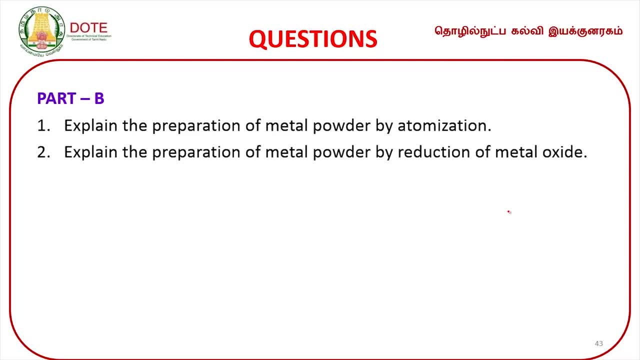 methods. they give the two marks. What are the possible? three more questions in this particular powder metallurgy lesson, Explain the preparation of metal powder by atomization. That means atomization method. how will you prepare it? We will ask only How will you. 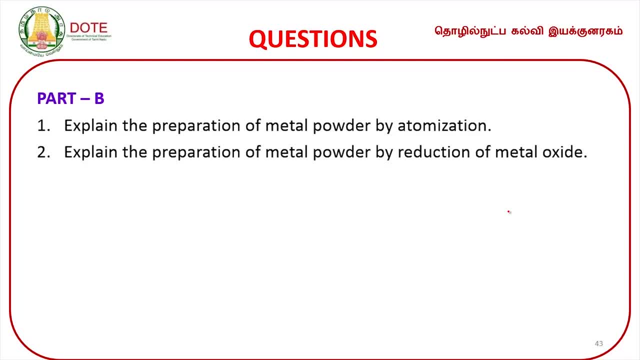 prepare the metal powder by atomization method. or sometimes we will ask what explain the preparation of metal powder by reduction metal oxides. So the examples we have, we are given a two examples. one is a reduction of what cupric oxide to copper. another one is a reduction of is tungsten oxide we will convert it to. 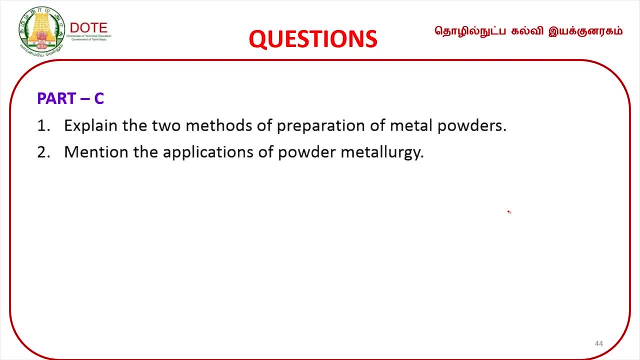 tungsten. So any one method, you have to explain the things. and in the five more questions we explain the two methods of preparation of metal powders. they are asking to write all the two methods. we studied about only two methods. one is a atomization method and 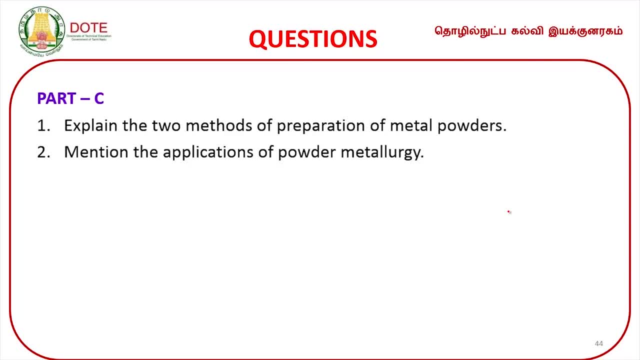 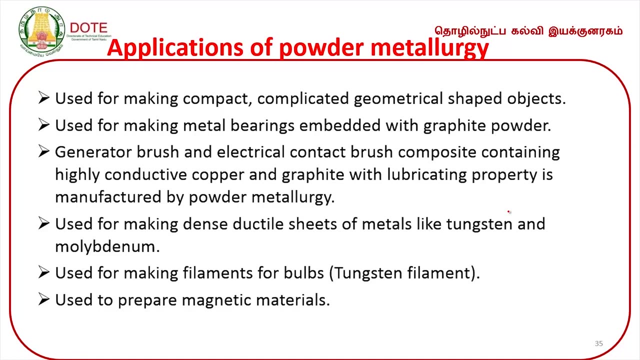 one is a reduction method. both the methods you have to write with equations and mention the applications of powder metallurgy. the applications of what? powder metallurgy? lot of application. we discussed. see that one used for making compact, complicated, geometrical shaped objects in the powder metallurgy with a applications, not only that one: metal bearings.